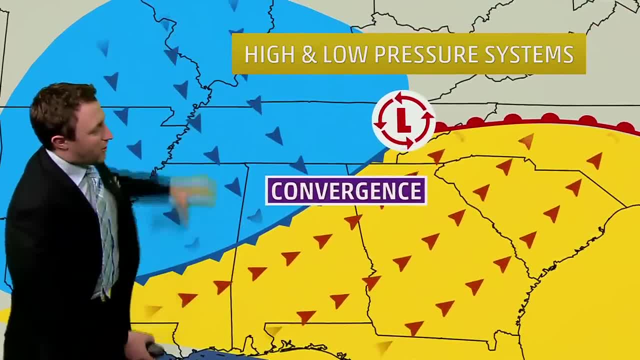 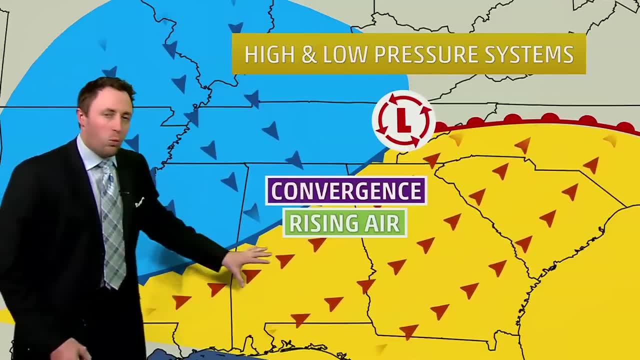 precipitation. what's going to happen here is you've got this air coming down from the north and this air kind of going towards the north and east. what happens is this piles up as it gets close to this warm air mass and it starts to lift. so where these meet, all that wind meets. we call that convergence. 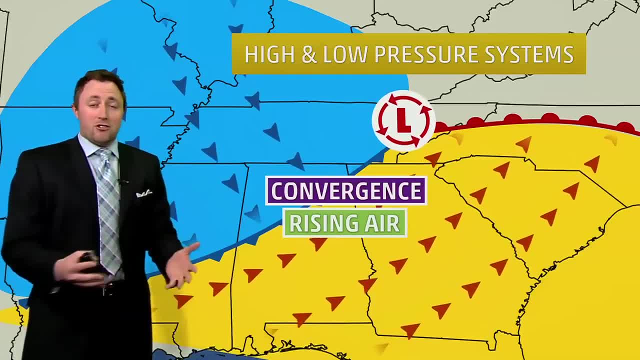 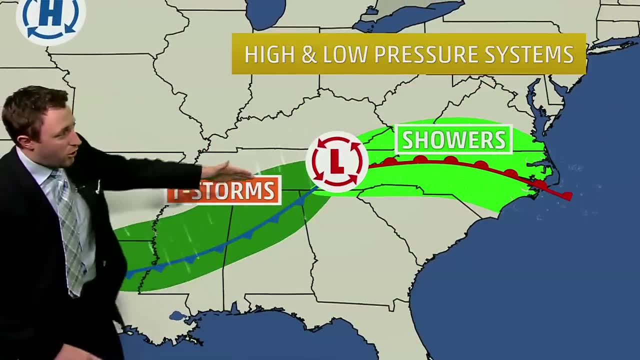 the meeting of air and when it happens, it starts to go. it has nowhere to go, so it has to go up, and once that starts going up, that's where we start to get clouds and rain, and usually along the cold frontal side of a storm is where we'll. 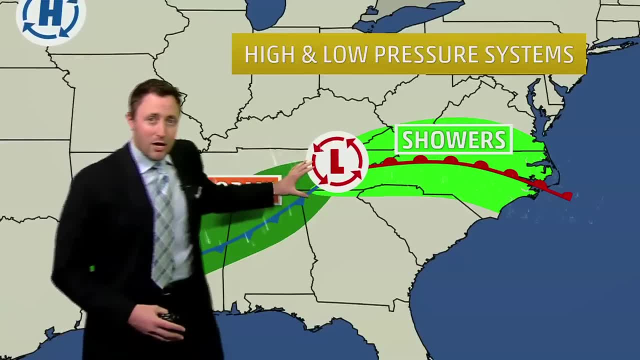 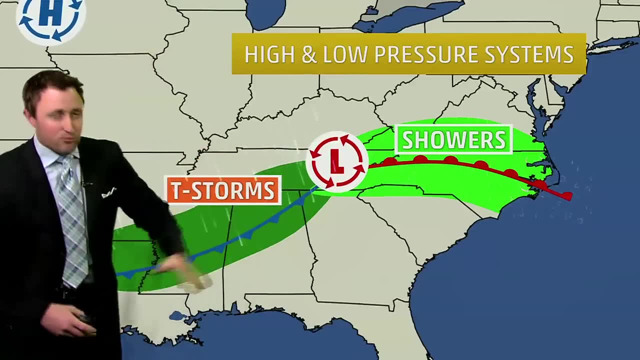 see things like thunderstorms. but on the warm frontal side over to the north, that's where we'll start to see just broad areas of rain and showers and cloudiness and as that comes through well, the weather gets a little bit cooler. Now high pressure, a little bit different high pressure systems, air goes. 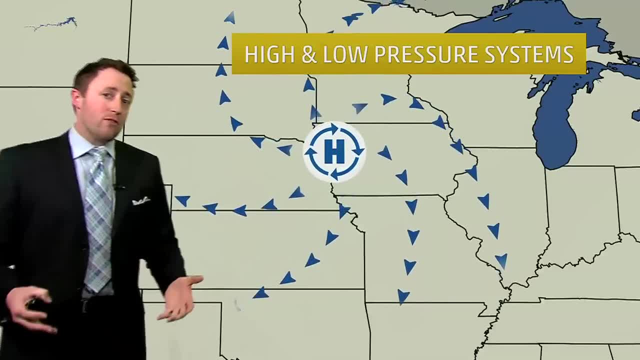 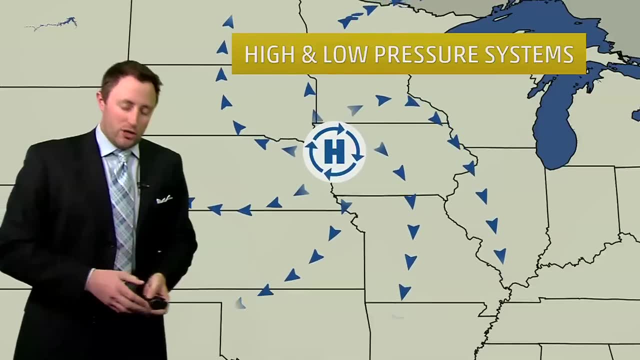 clockwise and outwards from an area of high pressure. so why don't we ever see any rain or anything near an area of high pressure? when you have all of this air moving outwards, it's actually like if you were going to turn the hose right on. 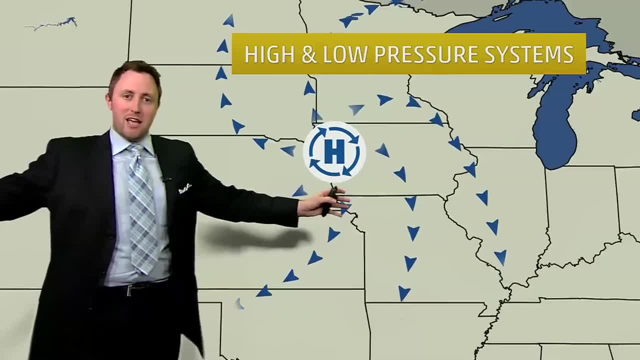 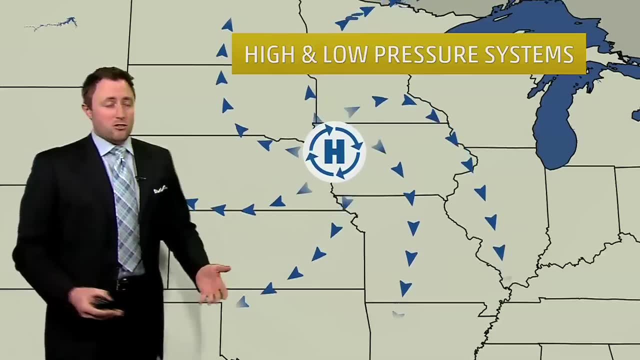 the ground. what happens is that water goes down and it spreads out. you don't have any lift, so you don't have anything to create that upflow of moisture, to create any precipitation. so usually when we talk about high pressure, we talk about nice weather. but let's take a look at what your forecast is. 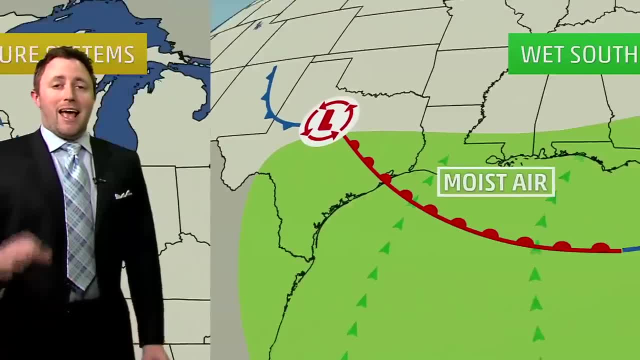 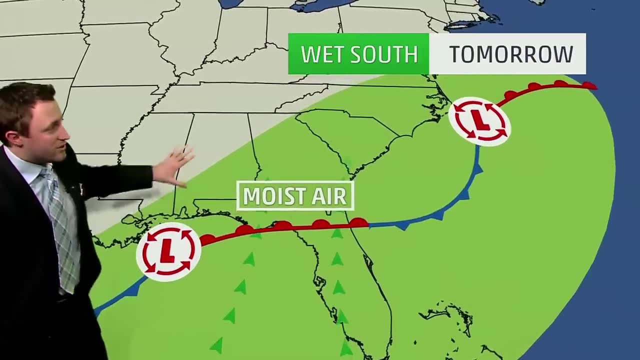 looking like as we go through the next couple of days we're going to be looking at a little bit of rain. we've got a couple of fronts to the south. here's our front. see the red with the half circles. that's going to come northward. we're going. 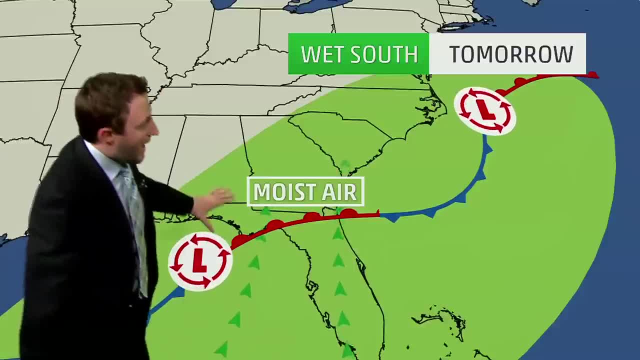 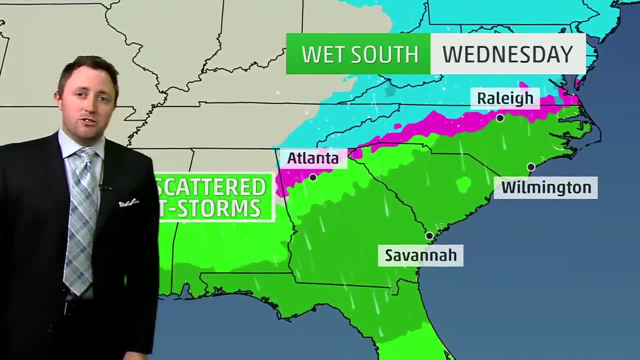 to see a little bit of rain in eastern and central North Carolina as these low pressure systems and their cold fronts and warm fronts move along the eastern seaboard. Then by Wednesday we'll see maybe a little bit of rain in Raleigh, but it quickly moves. 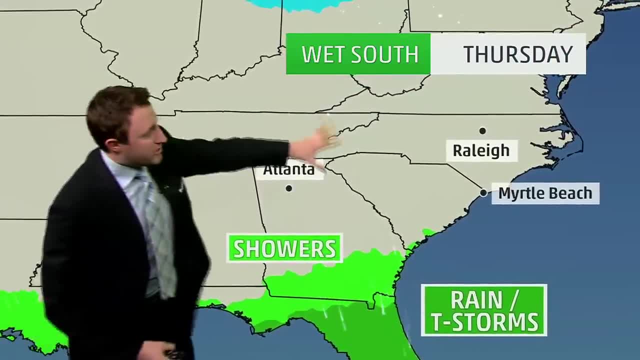 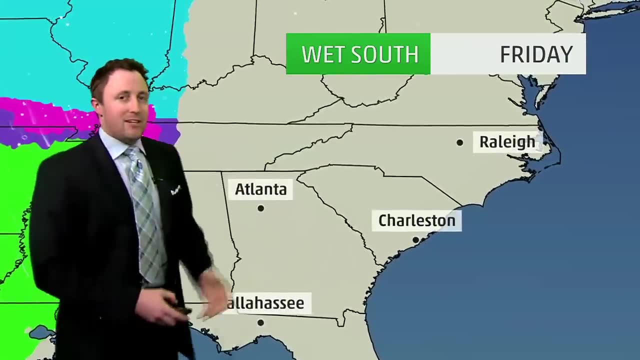 out and we start to see some high pressure move in. how do we know? Well, we don't see any weather going on here by Thursday and that'll stay the same even as we head into Friday. things kind of clear out, but the next weather system comes on in. we start. 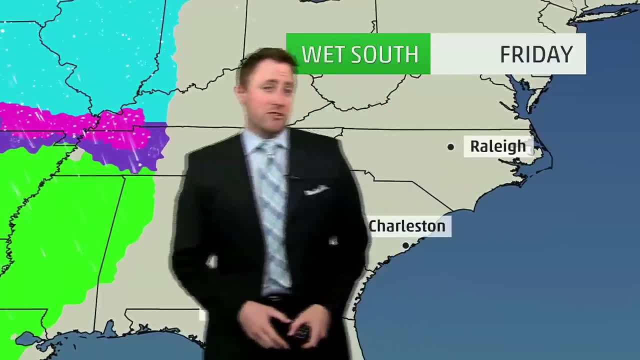 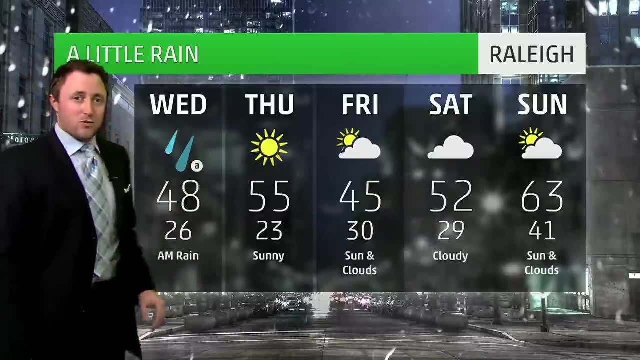 to see some rain heading in portions of western Tennessee and portions of Mississippi. So here's what comes up for Raleigh over the next five days. we've got rain on Wednesday and a little bit cooler. notice as we get that cold front to come through. it brings that.